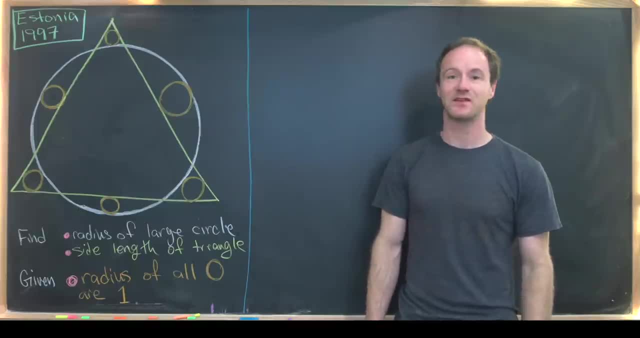 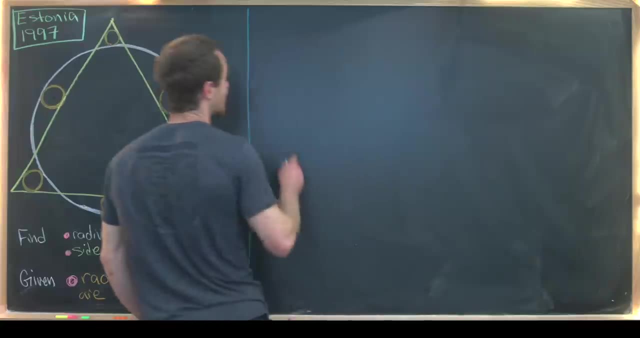 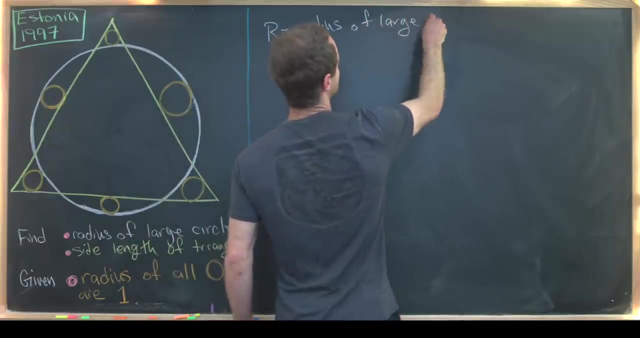 the radius of the large circle and the side length of the large triangle. So there'll be a couple of things that I start with here. First, I'll go ahead and set r equal to the radius of the large circle, so that we've got something to work with here. 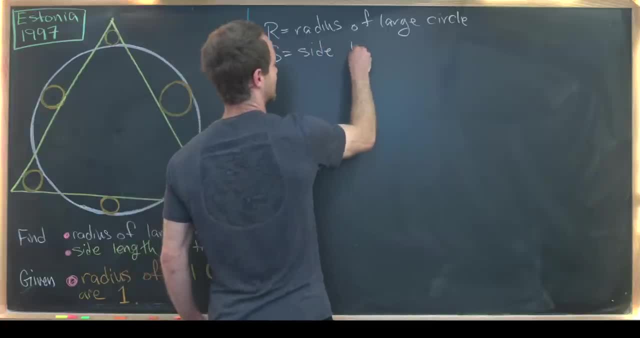 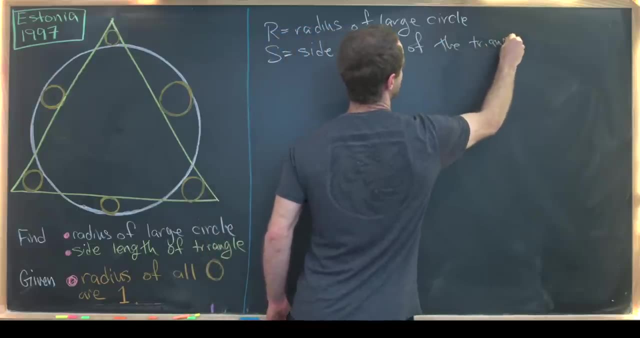 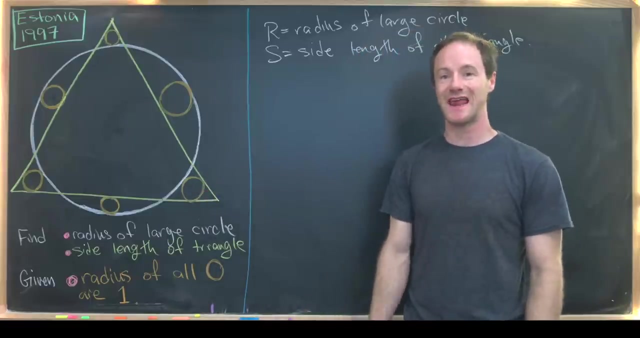 And I'll set capital S equal to the side length of the large triangle against r, And so we've got something to work with here. Next up, I'll notice that this small circle and the large circle are tangent, So that means, if I draw the tangent line, that they share. 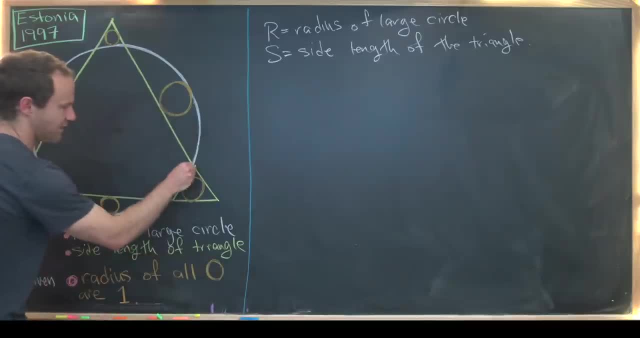 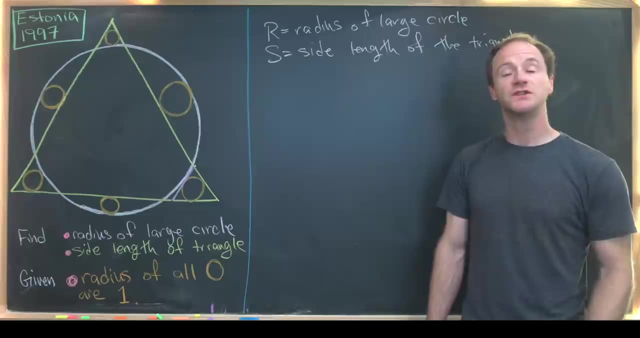 I create a sub-equilateral triangle in here. Maybe I'll make this purple so that it looks a little bit different. So that's actually going to be pretty helpful. So now we'll look at the general idea of our solution. I'm going to add some named points in here, So I'll call this one. 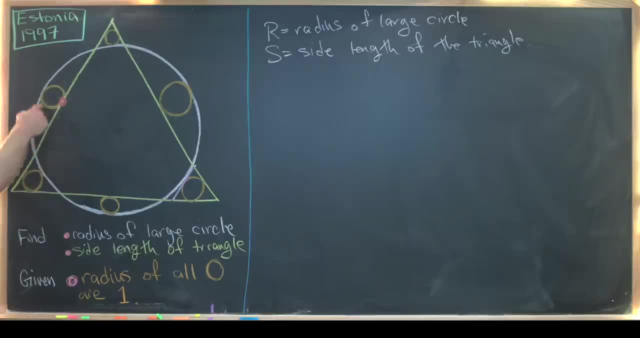 this point right here, which is the intersection of the large triangle and this orange circle, I'll call that B, Then I'll call this point over here, A, And then, furthermore, for good measure, I'll call this point right here C, And then the center of the circle. I'll call O, like for the. 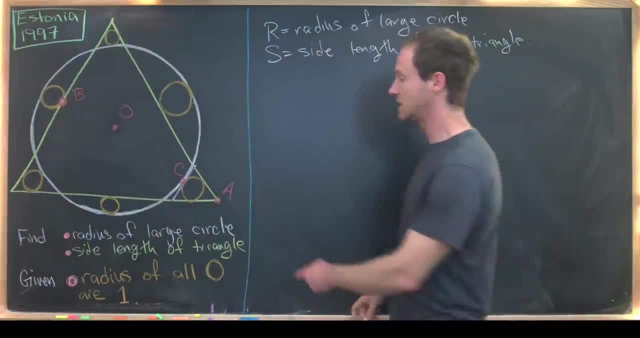 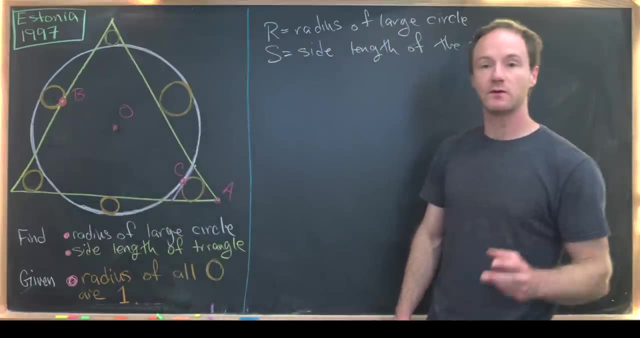 origin And essentially, what we want to do is measure the line segment length from A to B two different ways, And essentially what we want to do is measure the line segment length from A to B two different ways, And those two different ways will give us a nice system of equations that involves R and S. 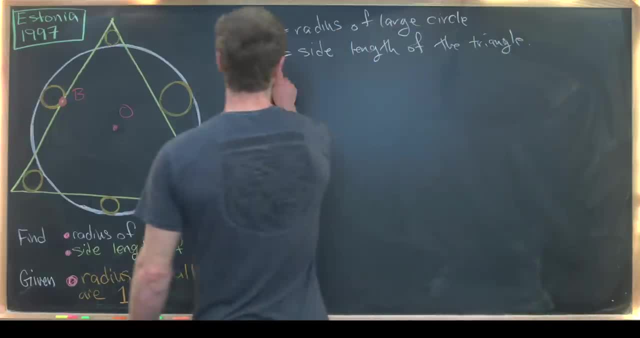 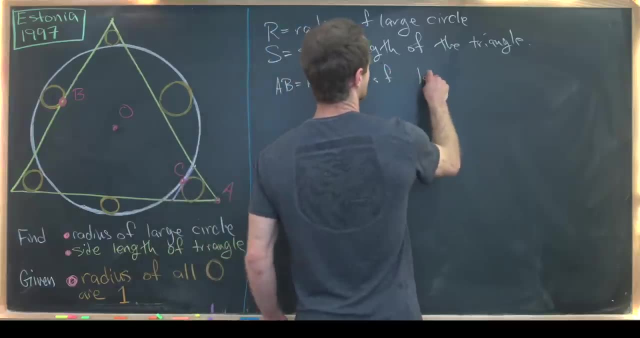 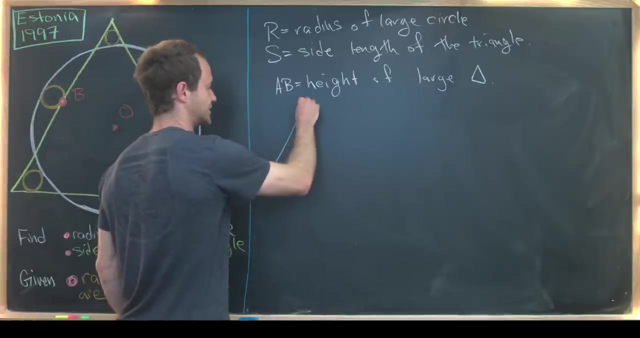 So the first way I want to do that is notice that AB is going to be exactly the height of the large triangle, So we can make a pretty simple calculation in order to determine that. So let's say this is our large triangle, with side length S. 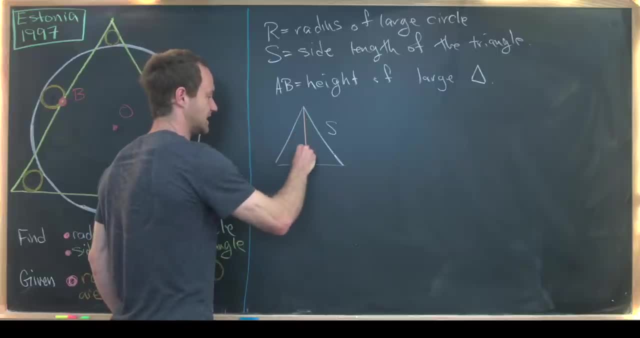 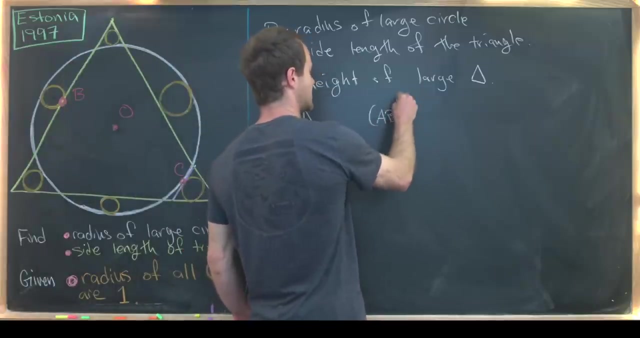 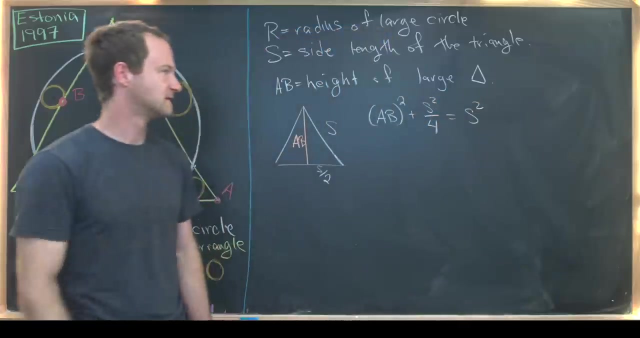 So this guy right here is distance AB. just by our picture here, That makes this right here S over 2.. Now we can use the Pythagorean theorem to find AB. So notice that length AB squared plus S squared over 4 equals S squared. Okay, but that tells us that the length of AB squared is equal to. 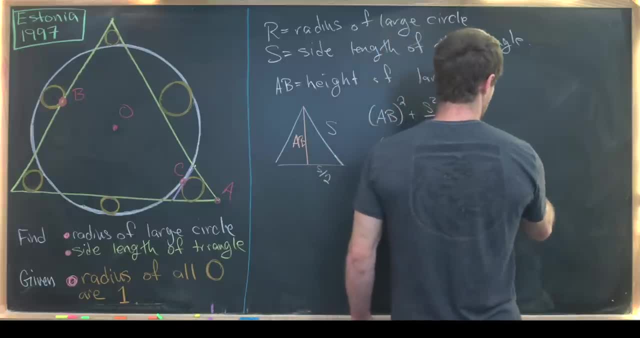 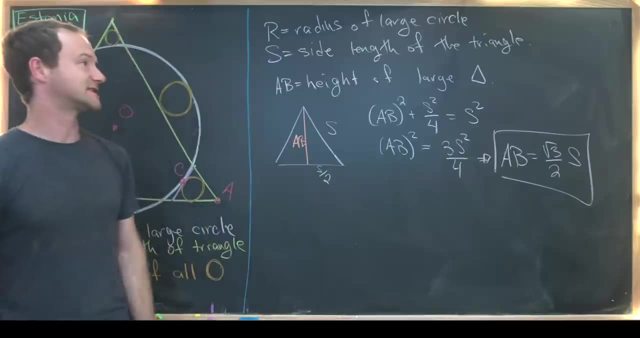 3 S squared over 4.. That means this length AB is equal to the square root of 3 over 2 times S, where S again is the side length of the triangle. Okay, so let's maybe take that information up here and then we'll measure AB a different way. Okay, so we just got done with our first calculation of. 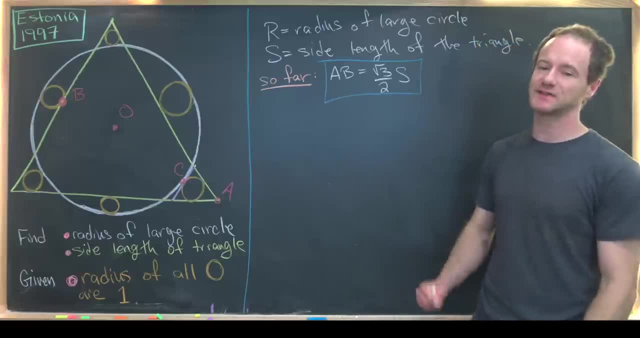 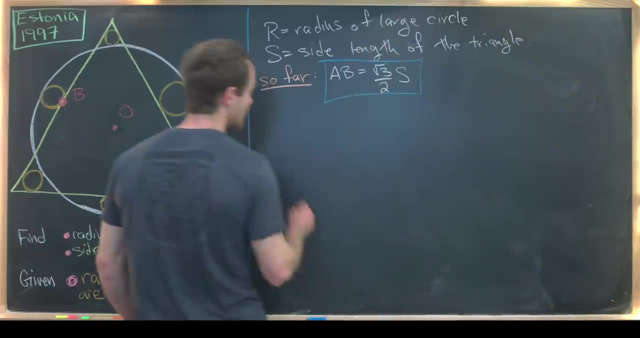 length AB. We found that it was root 3 over 2 S, where that was the side length of the large triangle. Now I want to calculate length AB b one more way. that'll be like this, so notice a b is also going to be equal to the length a c. 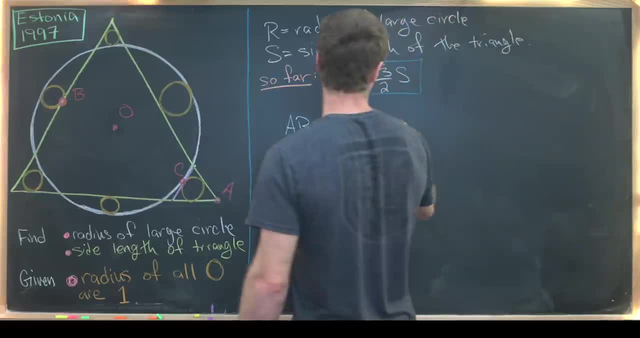 and then the length b c. so i'll just put plus b c here, but notice that's equal to length a c. and then b? c can be easily calculated because b c is the diameter of the large circle minus the diameter of one of these small circles. but we know the diameter of this small circle is. 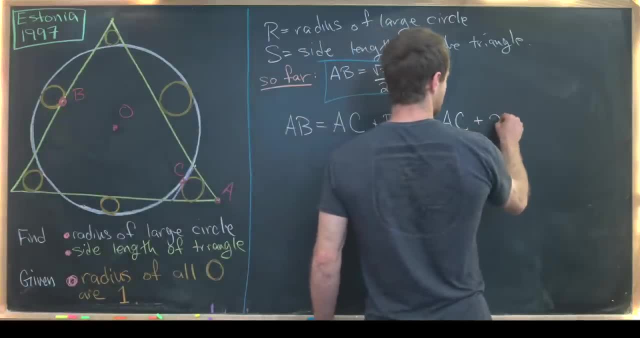 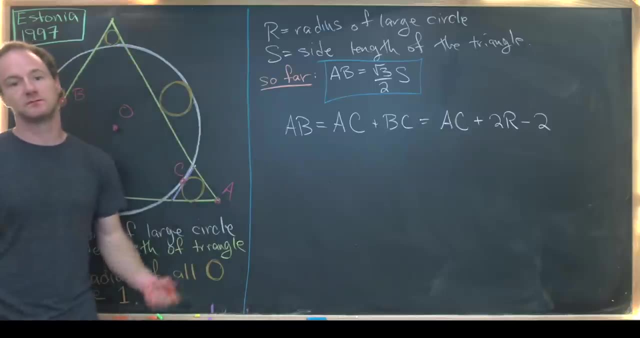 one. so let's see. like i said, it's going to be the diameter of the large circle, which is 2r minus the diameter of the small circle, but the diameter of the small circle is 2.. so now we just have to calculate a, c. so let's maybe expand this picture of this small triangle out here. 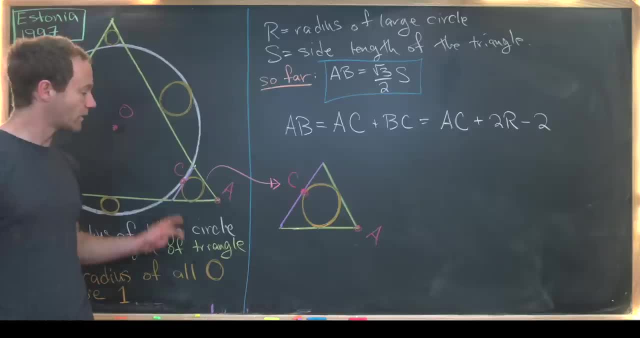 here so that we can calculate a c. nicely, okay. so i've expanded out this picture so that we can easily calculate a c. so notice, we don't know the measurement of this triangle, but we do know the measurement of the circle on the inside, in other words, the radius of the circle on the inside. 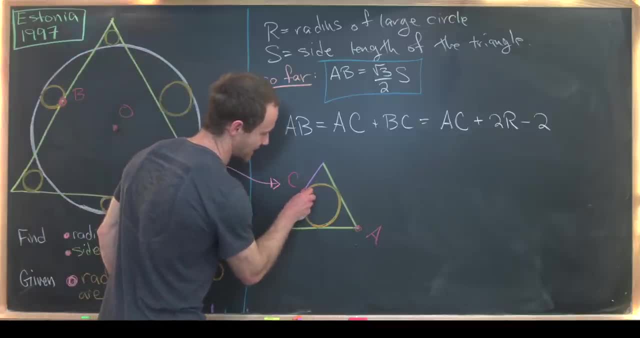 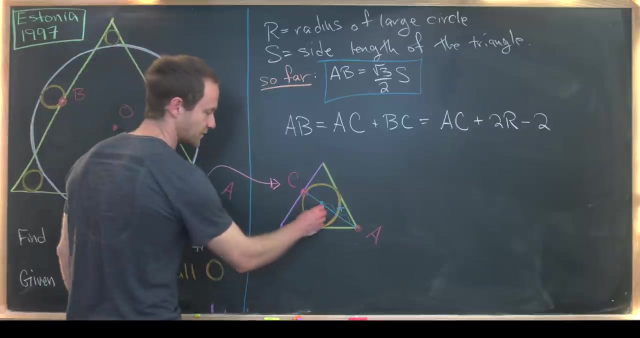 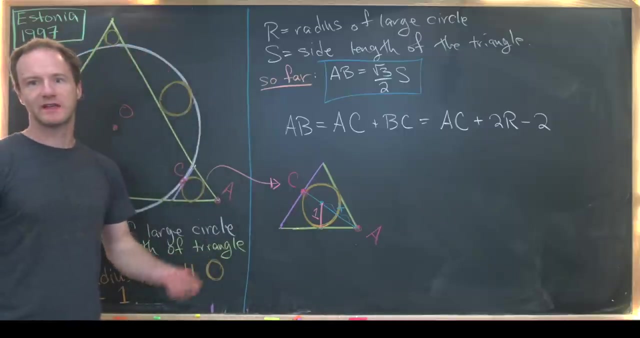 so we can use that to help us out. so i'm going to break this a c down into parts. i'll put the center of the circle right here, like that, and then i'll call over r equilateral triangle, so we know the measurement of this angle. that's going to be pi over. 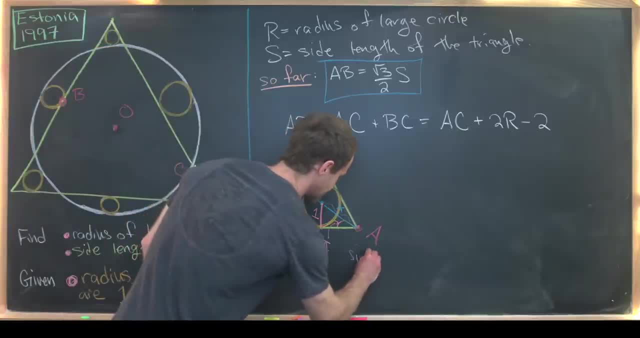 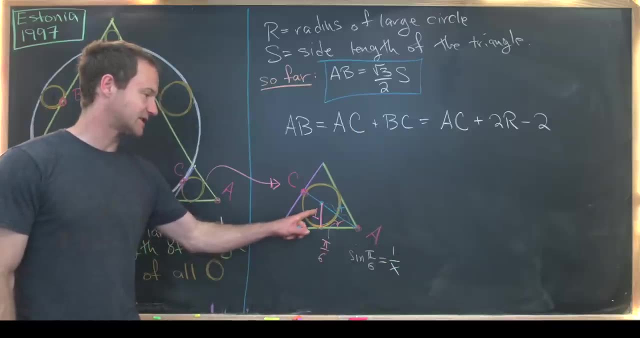 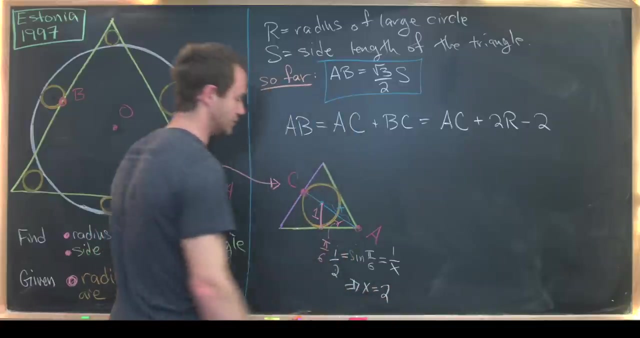 6. finally, we know sine pi over 6 going to be equal to 1 over X, because sine is opposite over hypotenuse. but sine pi over 6 is equal to a half, which means X is equal to 2. okay, but again we. 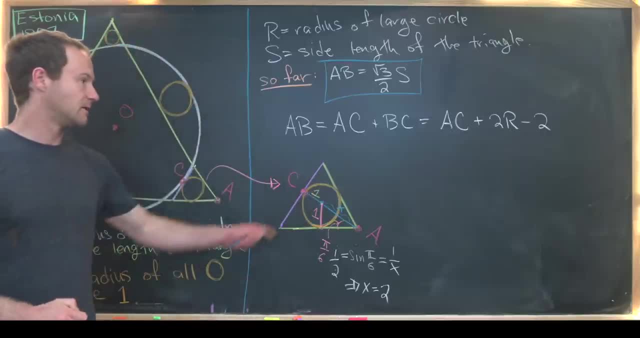 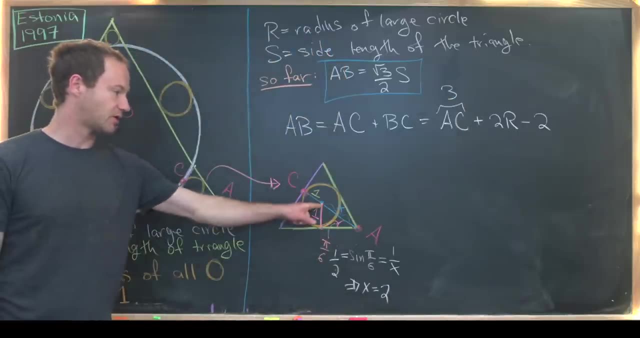 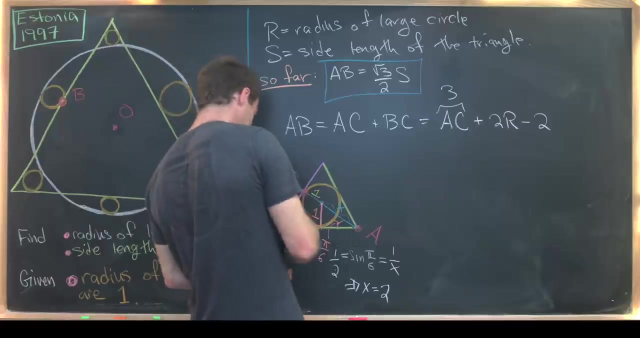 know that this is another radius of the circle, meaning that AC has length 3, because we've got 2 from this value of X plus 1 from this extra radius of the circle. so, putting this all together, we see that a- B is also equal to 2 R plus 1. 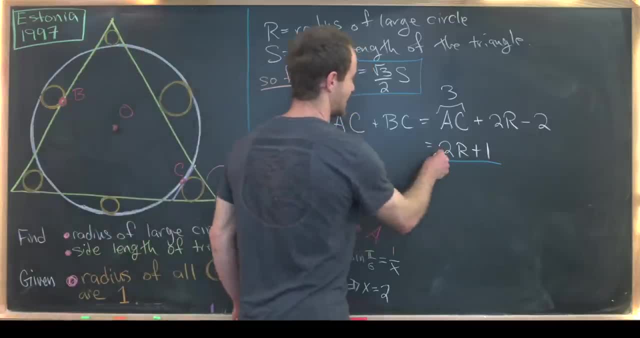 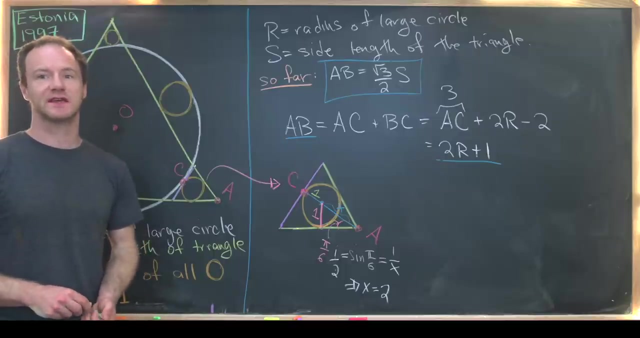 so that gives us another expression of a- B in terms of the radius of the circle, and in turn that gives us a linear relationship between S and R. so let's keep that linear relationship and then we'll find another linear relationship between S and R. so by measuring a, B, the distance. 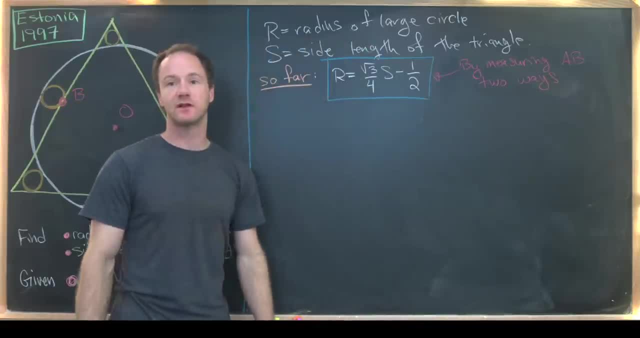 from this point to this point, two ways. we determined a linear relationship between R and S, so I've recombined it a little bit, and we found that R is equal to root 3 over 4 S minus half. now we're ready about to finish this off, so I'll 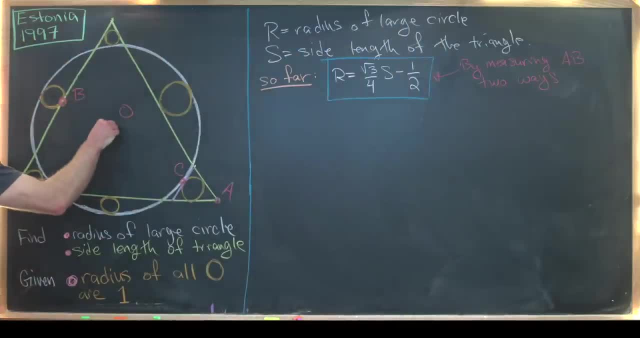 do that by introducing another right triangle into this situation, so it will go from here to here- maybe I'll call this point P- and then down through C to A great. now I want to notice that this length right here is exactly equal to S over 2, given the fact that P is pretty clearly the midpoint of this bottom side. 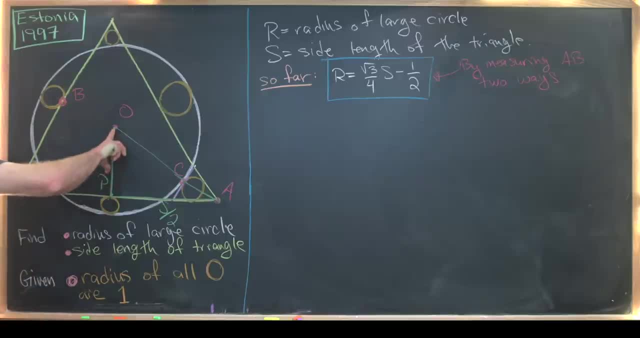 of the triangle. next, we can measure this distance from O to P pretty easily as well. so notice that is going to be equal to the radius of the circle minus two units, because we've got this small circle here, so I can put: this is equal to R minus two. then we can also easily calculate this length. well, what's?